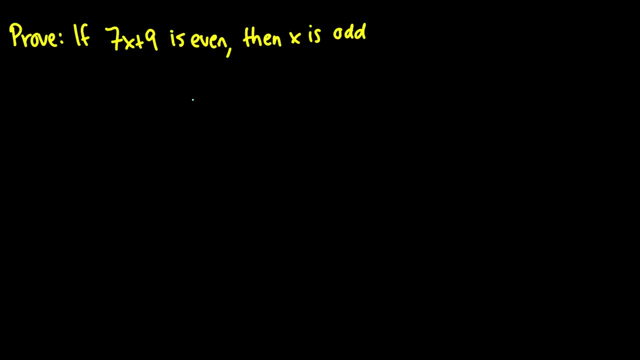 Well, that is just ridiculously hard. So we can make this so much easier. Why don't we say, okay, if not x is odd, then not. 7x plus 9 is even. Okay. And we know this is the same thing as saying if x is even, then 7x plus 9 is odd. 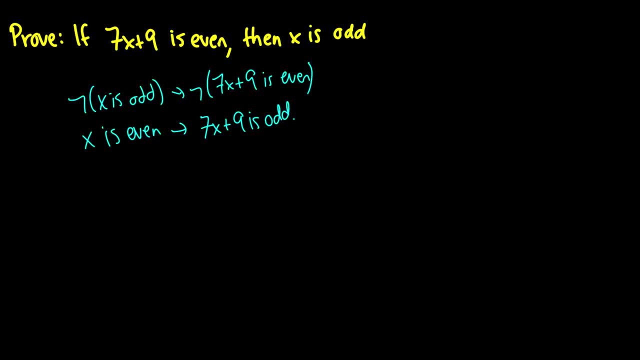 Okay, Well, I could do a proof here, a nice mathematical proof. but it should be obvious that if x is even, then 7 times x is even, and then an even plus an odd is going to be 7x plus 9.. 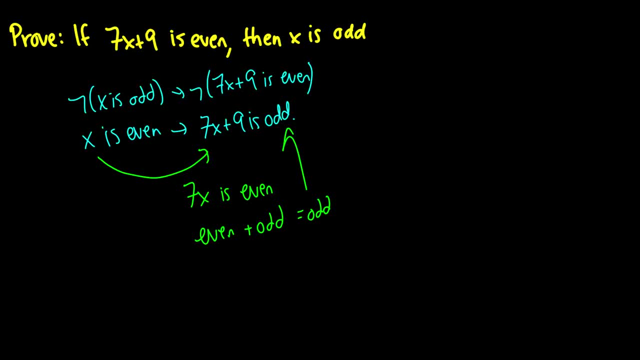 Okay, Okay. So if 7x plus 9 is even, then 7x plus 9 is odd. So we've just proven that 7x plus 9 is odd. So I'm being a little bit lazy with my proof there, but it's more to show that, hey look, this proves the exact same statement. 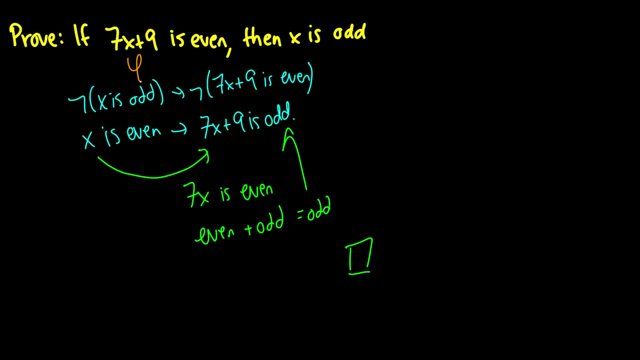 I'm saying: okay, let 7x plus 9 be phi and let x- is odd- be psi. Okay, now I'm going to prove: not psi, arrow, not phi. So what you do is: you assume not psi, Which is what I did here. 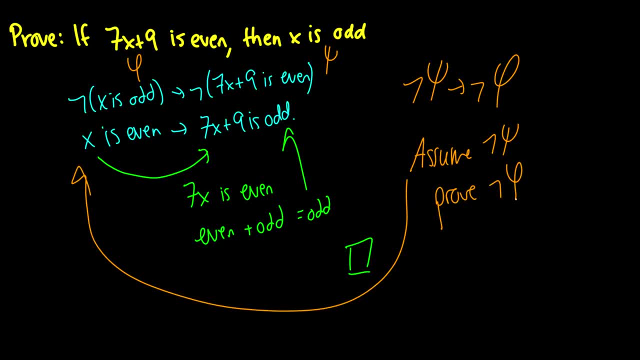 And then we prove not phi, which is what I did there. So really not too bad, In fact a little bit easier than doing it in a direct proof. Now I have this blank page for one reason, and one reason only. 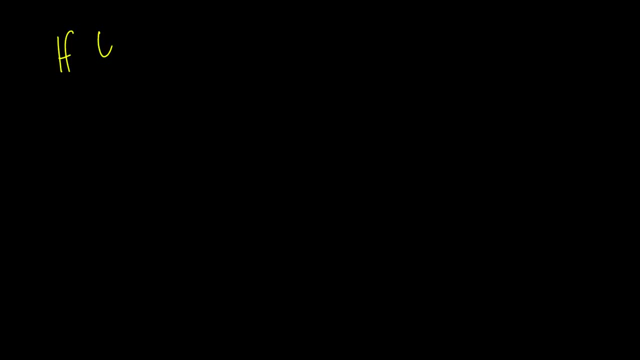 So if If phi or psi, then chi, Suppose I want to do a contrapositive proof on this- Then I have: if not chi, then not phi or psi, Which happens to be: if not chi, then not phi and not psi by the Morgan's Law. 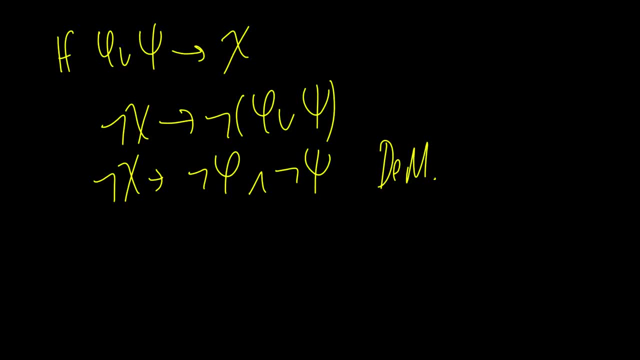 So a common error here is that You just prove one of these and you say it's conclusive. Really it's not. You have to check that both of those are negations And of course this is a logic thing. 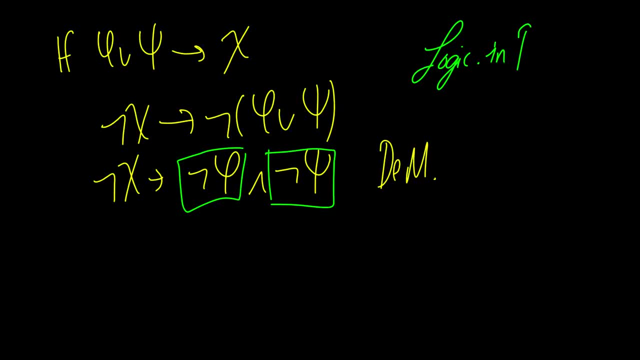 But in proofs it is still very important that you have your logic correct. That's why we did logic first, So this wasn't exactly too bad. However, Consider the case where I Say if phi, then not chi and psi. 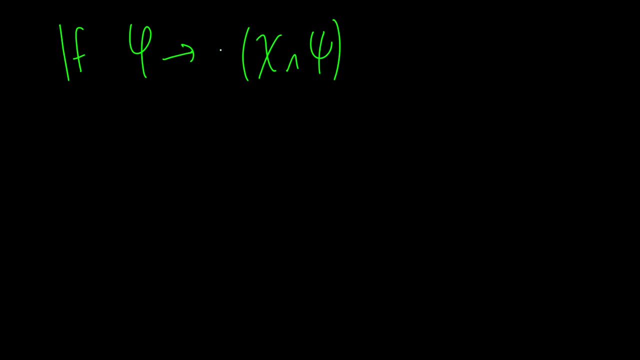 Or rather, I'll just say: if phi, then chi and psi. Okay, So if we assume phi, then we should be able to get both of these. However, if we have a contrapositive proof, what's interesting now? 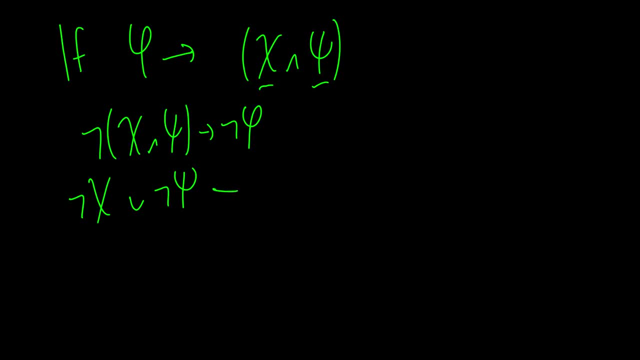 Is we get this nice Logical equivalence And when you have an OR statement, This becomes a proof by case. So you have to be very careful when picking your proof method That you make sure the logic works, Because here we have to have a proof one. 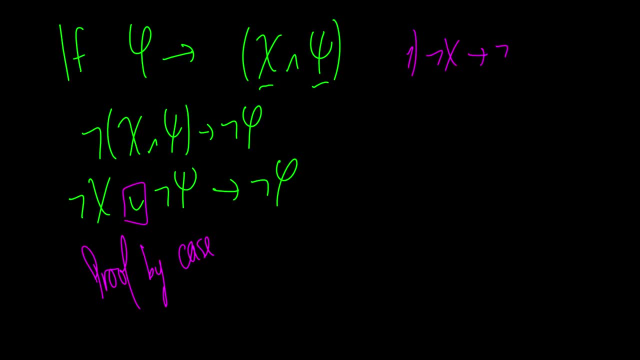 That starts with not chi and gets to not phi, And then you have to have another proof that starts with not psi and gets to not phi, And only then can you conclude not phi. So be very careful with your logic. I know this is another fast video. 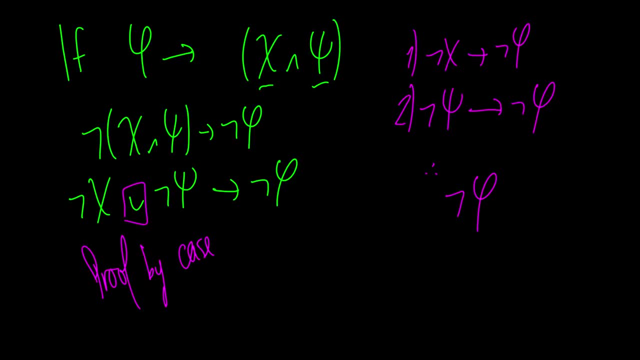 But the point is to show proof methods, not proof examples. I do give you one example in each proof method, But this one is special in that the logic is very, very important to take care of. In fact, that's why most of this video is based on the logic. 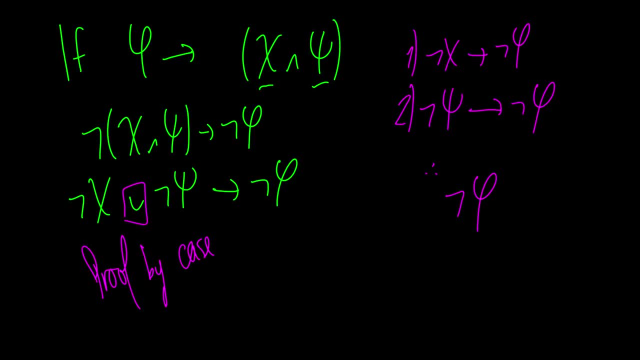 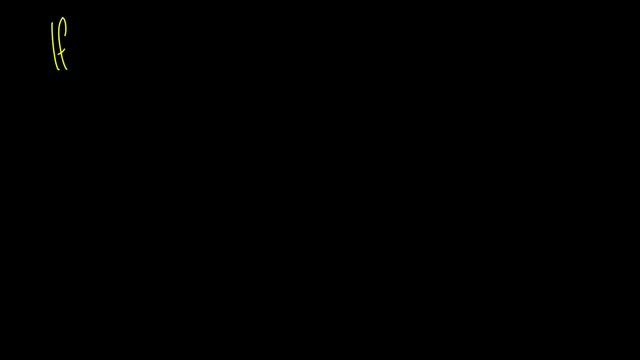 As opposed to the actual proof method. So as an example- And I will give an example of this here- Let's say if In fact this isn't exactly a nice mathematical proof, This is sort of an everyday, you know, kind of fun proof.